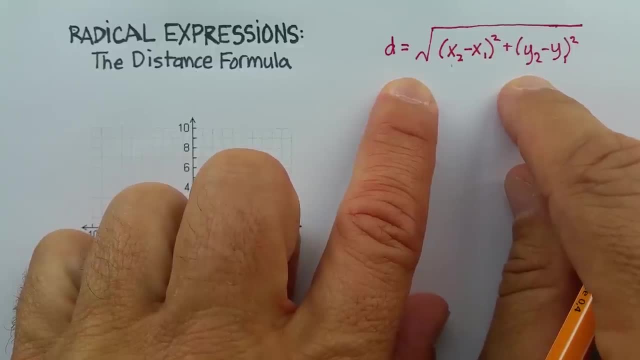 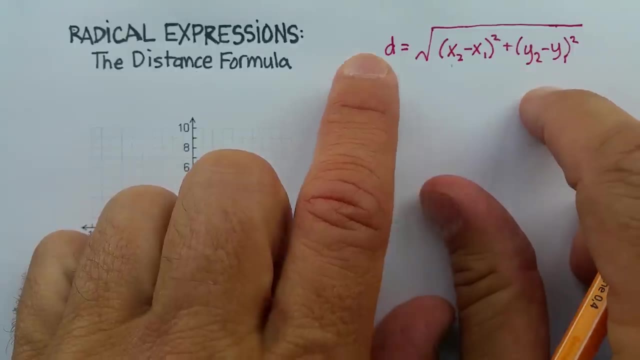 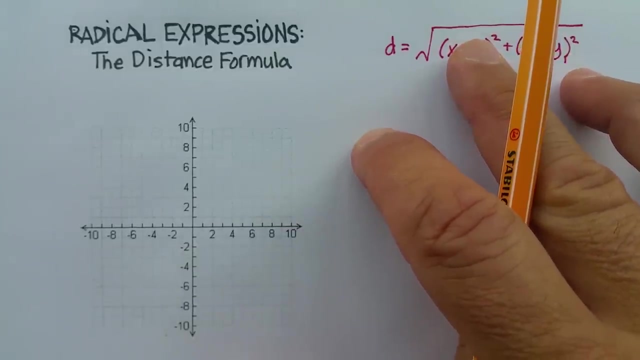 because this distance formula is used a lot in geometry, especially when you're trying to find triangles or distances on a side of a triangle, that sort of thing, or just really any odd-shaped polygon. Now let me show you how this works. 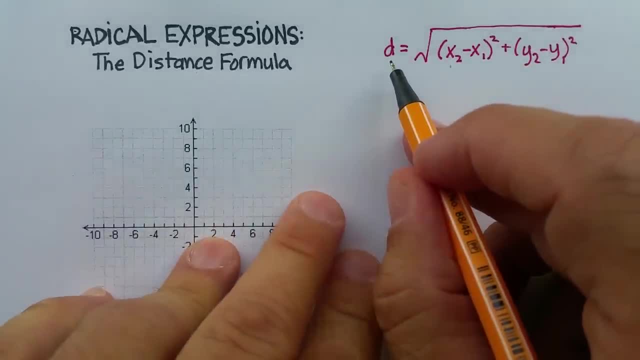 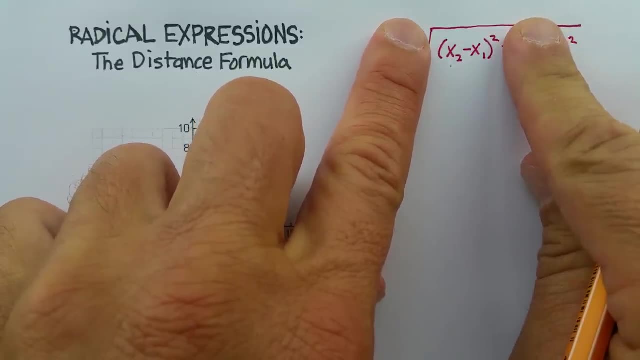 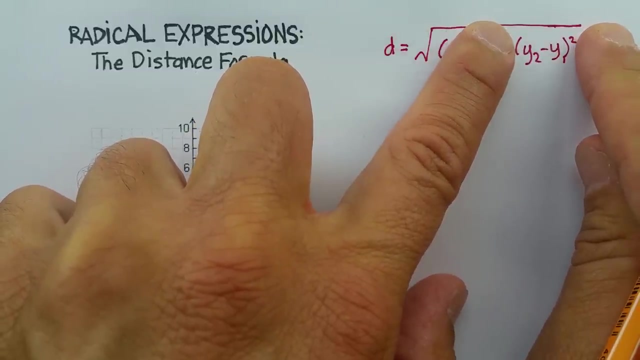 So the formula itself is that the distance between two points is equal to the square root of the difference between the two x's and the coordinates of those two points squared, plus the difference between the two y's Of those same two points, again quantity squared. 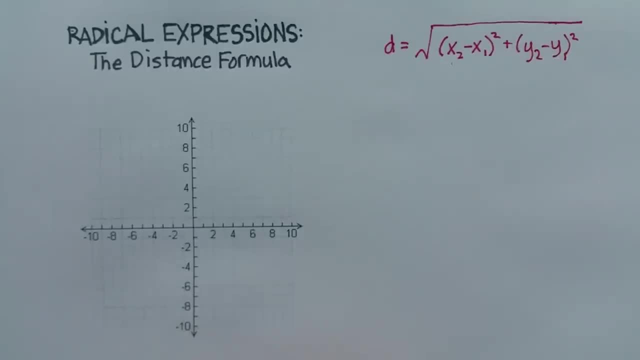 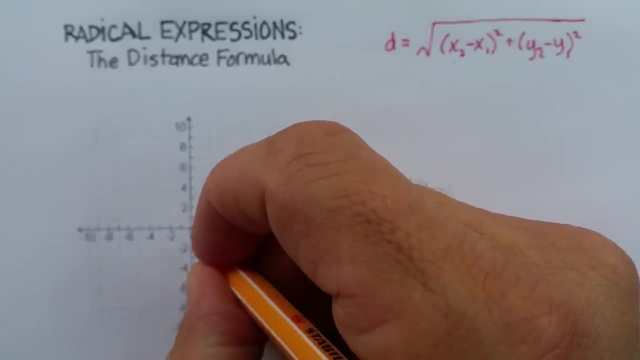 Now what does that mean exactly? Let's just see an example of that. Now, over here I have a coordinate plane and let's just pick out three points. okay, I'm going to pick out three simple points. Let's just go with 0, 0.. 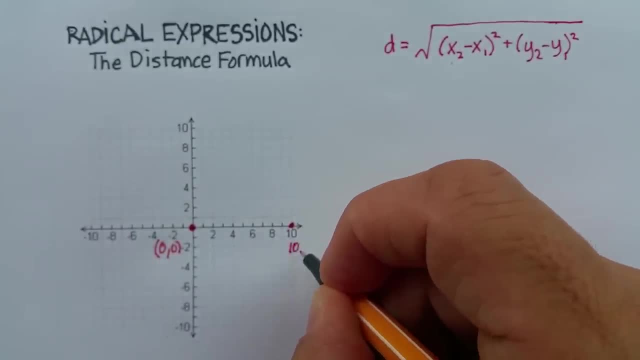 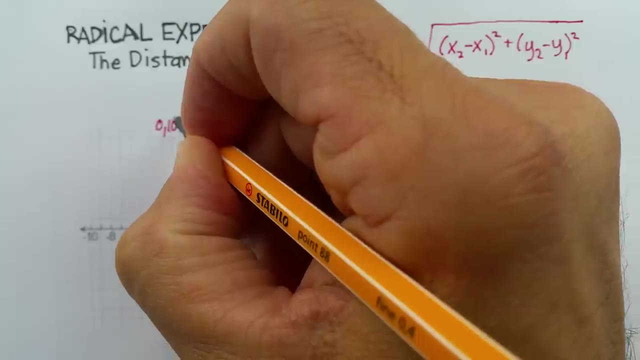 Let's go with this point here, which is 10 along the x, 0 along the y, And let's go with this point up here, which is 0. 0 along the x and then 10 along the y. right, 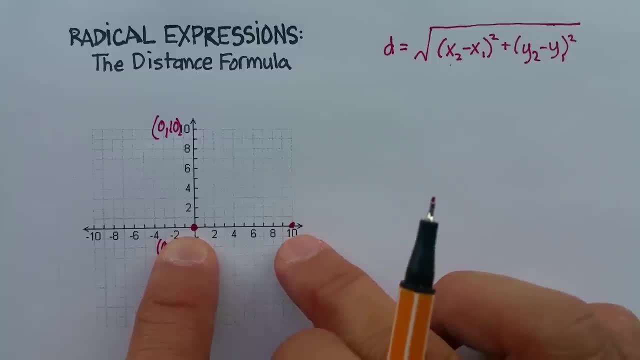 Now, if I wanted to find the distance between this point and this point, all I have to do is count along the x-axis: 1,, 2,, 3,, 4,, 5,, 6,, 7,, 8,, 9,, 10.. 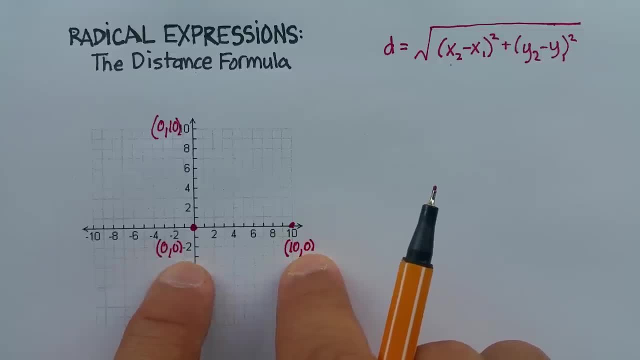 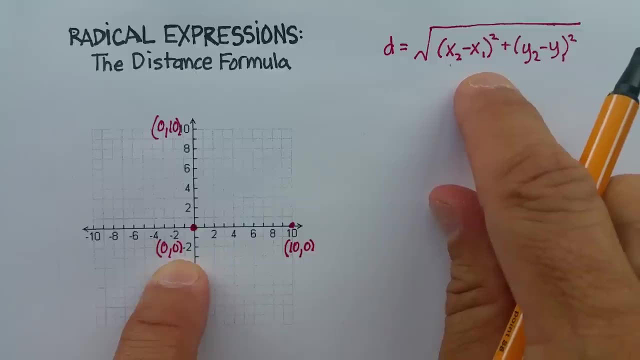 Sure enough, and it would be the difference between the x's, wouldn't it? The distance between the two 0's is just 0. So, filling it in here, it would be 10 minus 0. Which is 10 squared right. 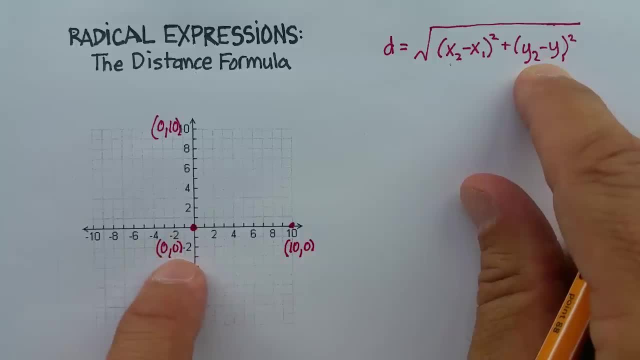 Plus, this would just be 0, because there's no difference along the y's right. So you'd get 10 squared, which is 100.. The square root of 100 is 10.. The distance, therefore, is 10.. 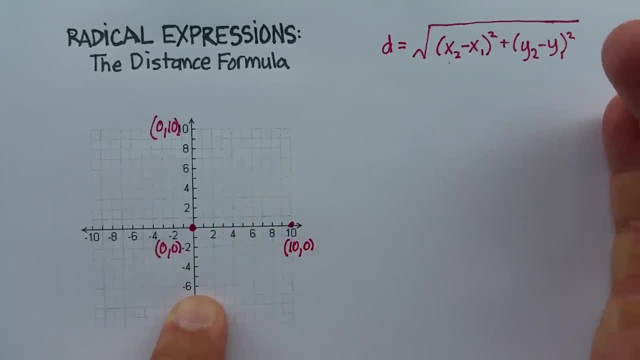 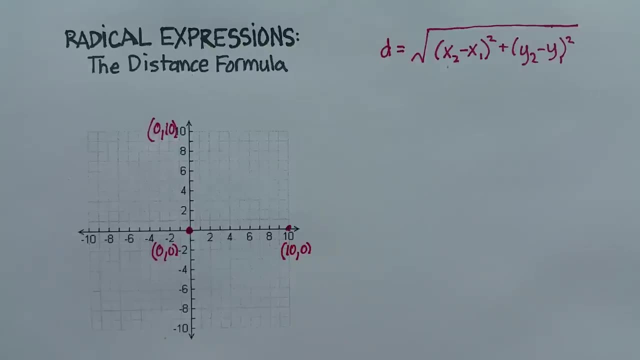 Or you just count the number of units, right, And there you go. Same thing would happen if we do the y's. I'll let you go ahead and do that on your own. But here's the question, right, What about the distance between this point? 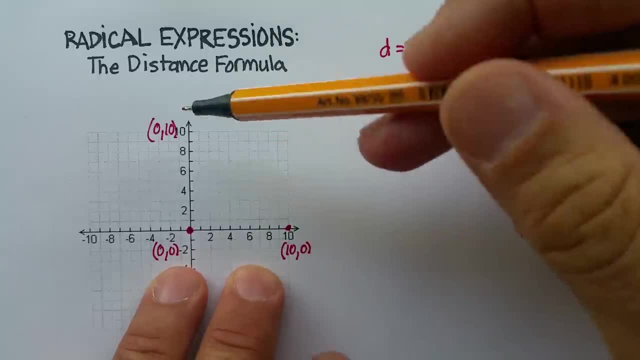 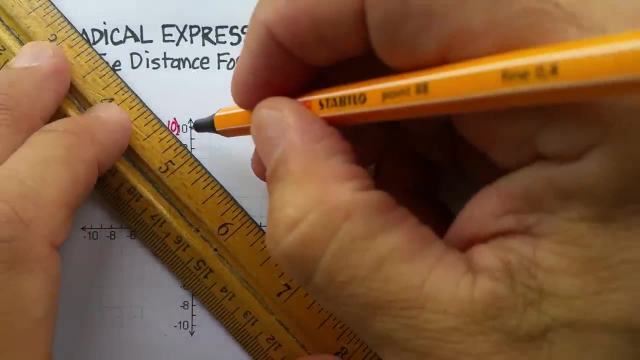 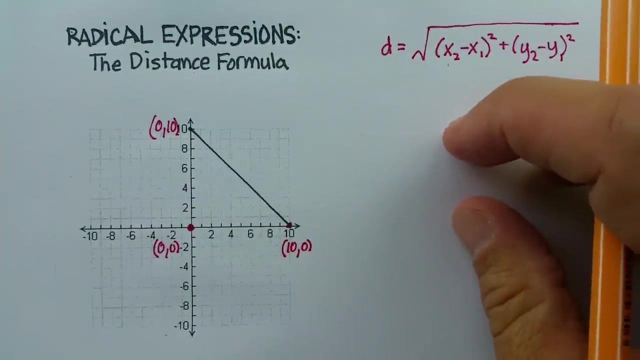 and this point. Notice that it's on the slant here, or the diagonal. Let me just draw that in here real quick. Okay, So what is the distance between that point and that point? I can't just count the number of units over, because it's increasing in size. 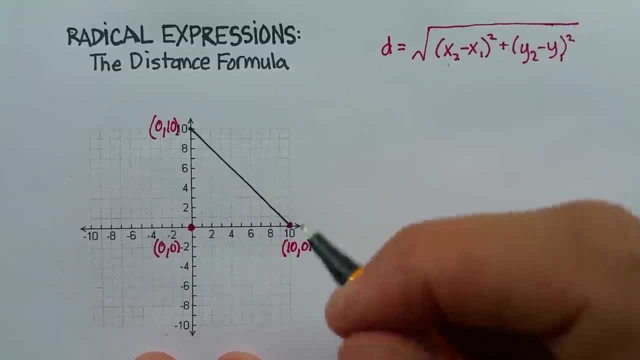 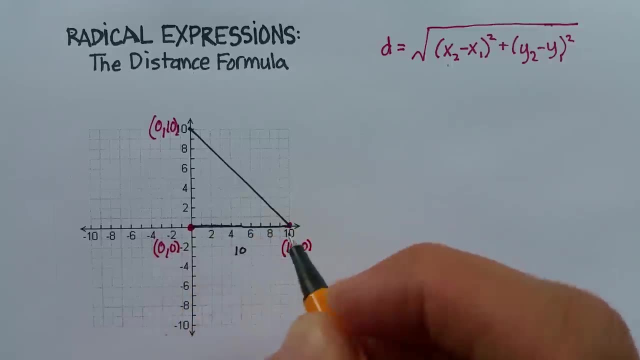 So that's when this distance formula becomes very important. Now, by the way, I'm just going to put, I'm just going to complete this triangle And say that we know that that distance was 10.. We already knew that that distance was 10 units, right. 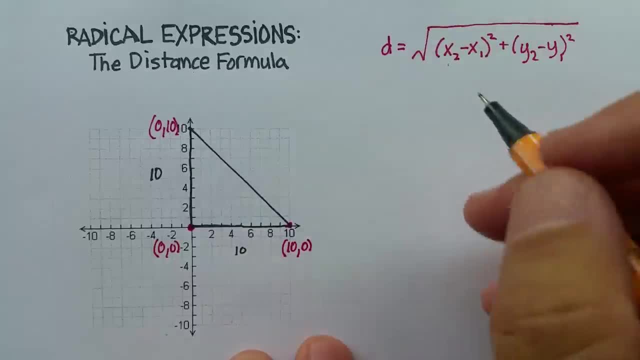 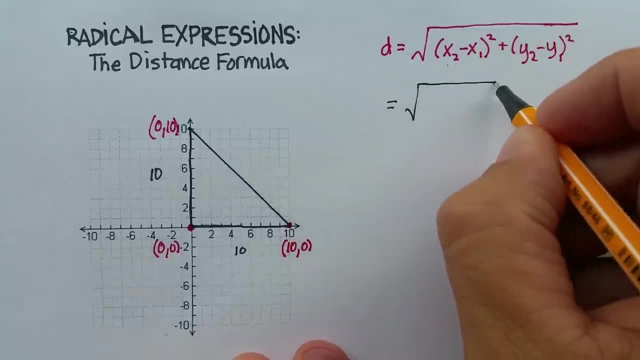 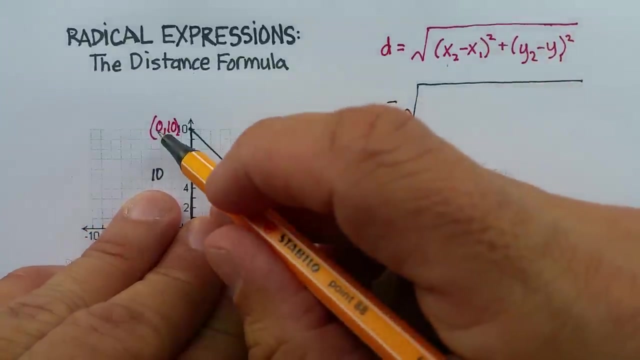 And now we're trying to find the distance of that one. So according to this, the distance is going to be equal to the square root of. let's just take the distance between two of the x's. So the x values here would be what? 10 and 0.. 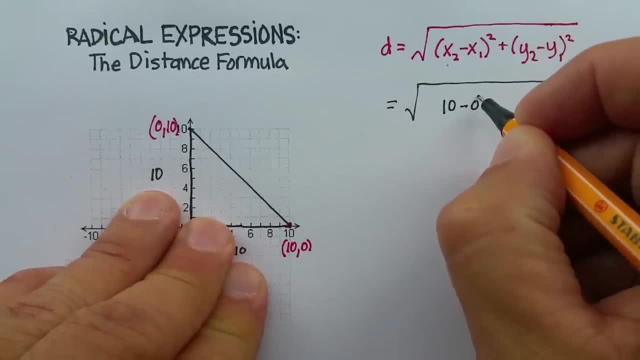 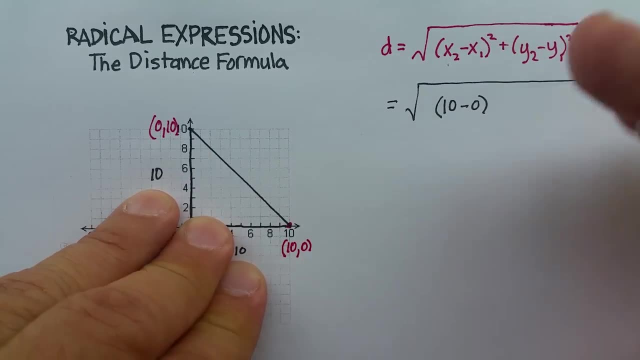 So let's just go 10 minus .0.. Now notice: this says x2 and x1.. It really doesn't make any difference which one's the x2 and the x1 is. As long as you've got the distance, the difference between the two x's, you're going to be okay. 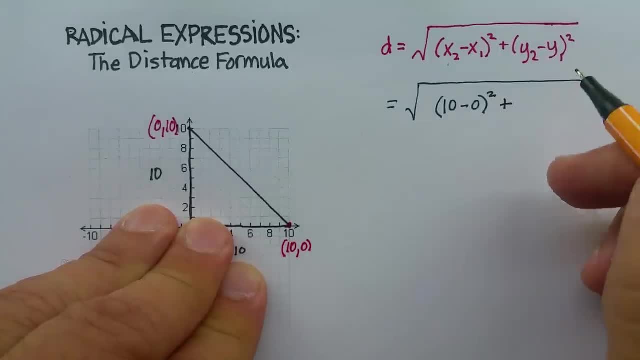 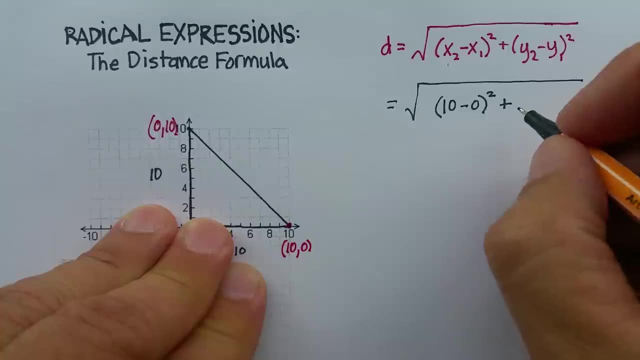 And that's going to give me. and then quantity squared. Now let's find the difference between the two y values, And it's 0 minus 10.. I'm just trying to keep them in the same order, So 0 minus 10.. 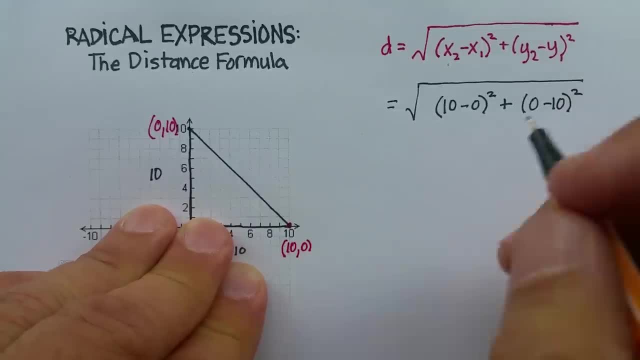 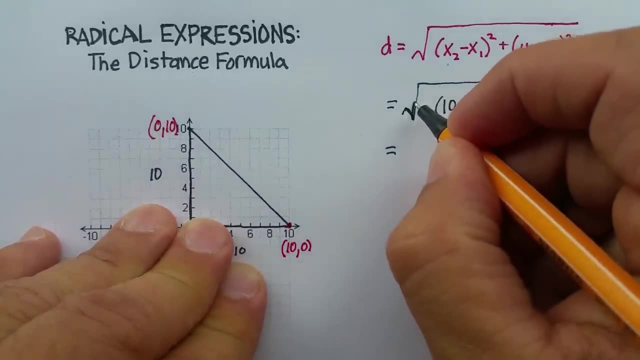 Again, .0 minus 10.. Again, quantity squared. Now let's just follow PEMDAS really closely Now. one thing to remember is that the radical sign is actually a grouping symbol itself, So it's like a larger grouping symbol. 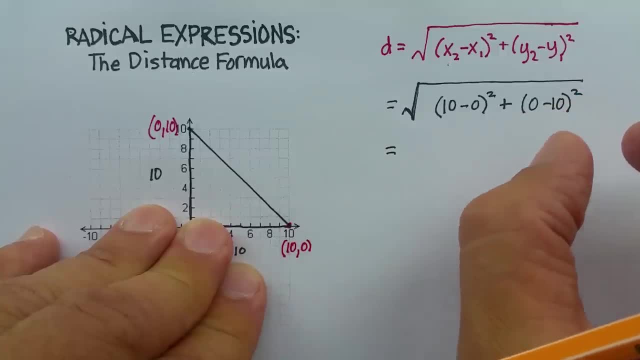 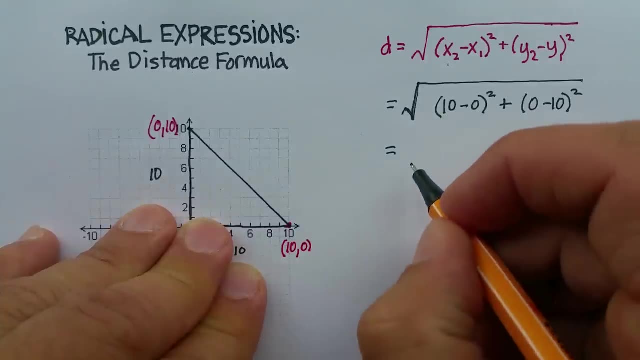 And in PEMDAS you're always supposed to go to the innermost grouping symbols first and work your way outward right. So the innermost grouping symbol is 10 minus 0.. That's just going to give me 10.. 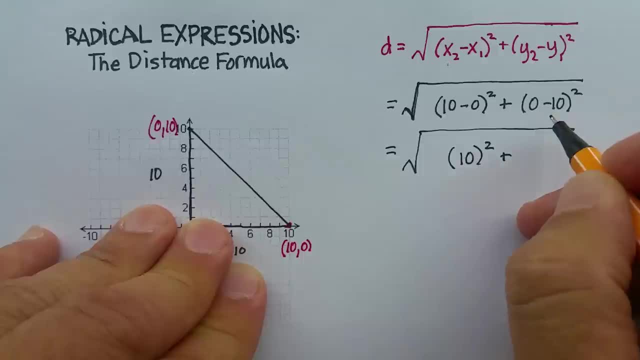 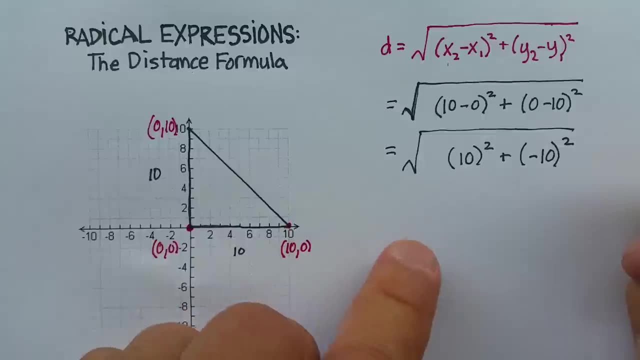 And then again quantity squared. Innermost grouping symbols 0 minus 10 are negative 10.. Again, quantity squared. Again, according to PEMDAS, you're supposed to move to the exponents now. So we've got. 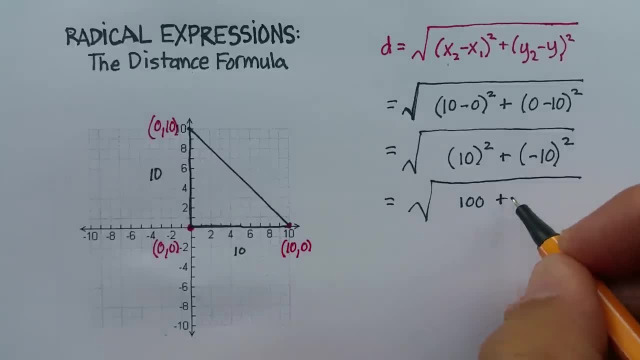 10 squared is equal to 100.. Negative 10 squared is also equal to 100.. Now I can go to the additions and subtractions. Here we have an addition Square root of 200.. And we know from our radicals that we could probably either do one of two things.